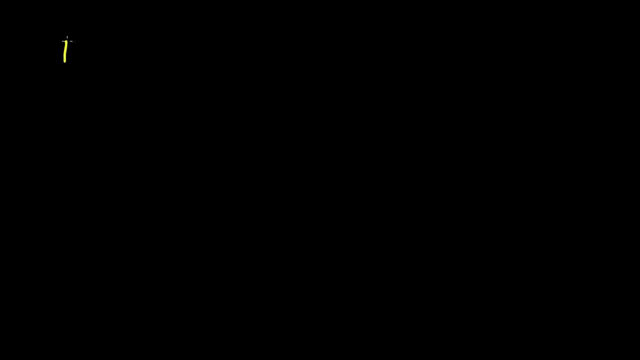 simplistic model of the internet would look something like this: We would have a bunch of PCs. We will say that this is a Windows PC and we will say this is a laptop. I will draw it a little differently. It is a pretty good looking laptop and, I don't know, maybe 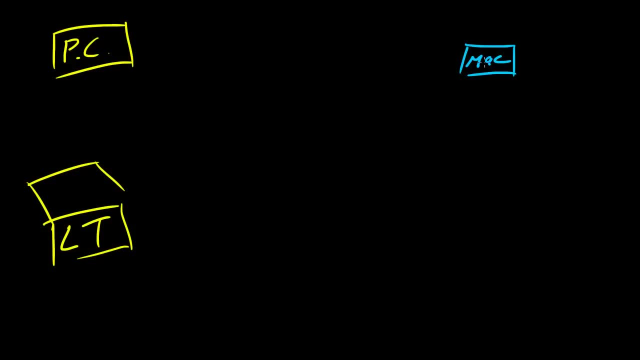 we have a Mac over here, Alright, and I don't know, maybe a Macbook later or somewhere else or something like that, but basically all of these things. you may hear them referred to as workstations. Workstations are basically home computers, laptops, Macs, whatever you. 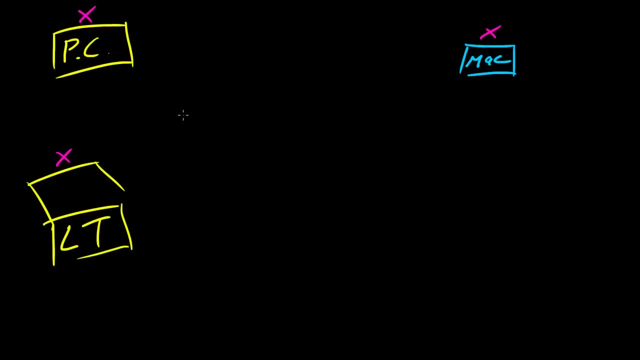 want to call them. Now we already know, aside from that, that servers- let me get a good color for it- servers are special computers. We will say that this is a web server. We will say that this is my server for my website, The New Boston, TheNewBostonorg. Now, believe it or not, my web server is actually. 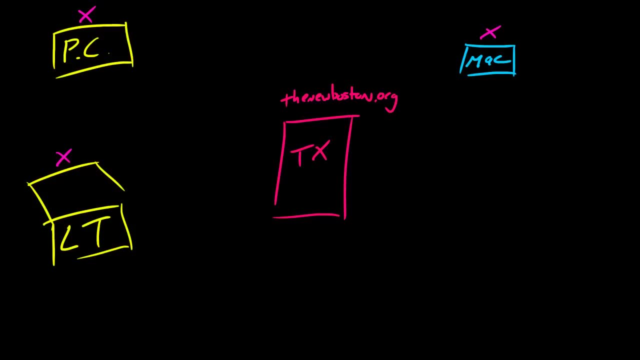 in Texas. There is a special computer in Texas that is storing all of my web files. so whenever you go to TheNewBostonorg, basically what is going to happen is this server is going to give you some files. So let's go ahead and talk about that process right now. Say: 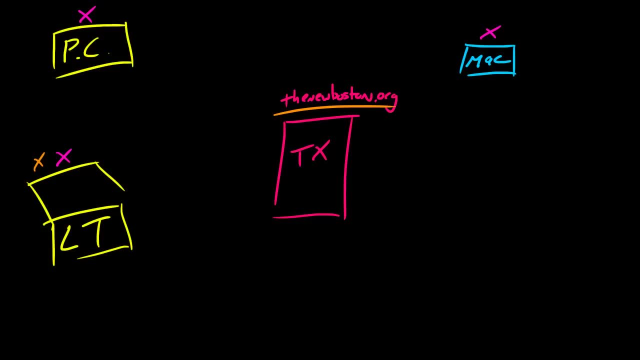 that this is you and you are watching this YouTube video on a laptop right now. Now you decide that you want to go to my website because you heard about it in this video and you want to check it out. So, basically, what you are going to do is you are going to type in TheNewBostonorg. 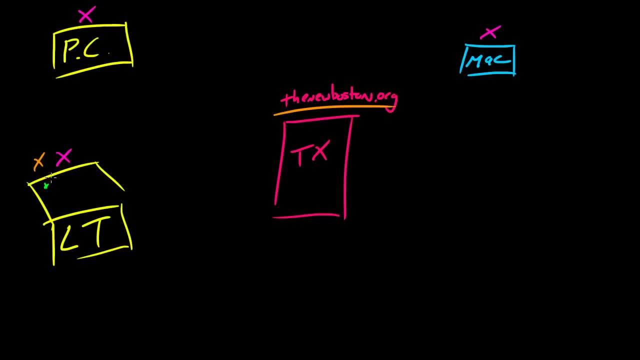 in your browser. hopefully you are using Google Chrome, So you are going to type in TheNewBostonorg and your browser is basically going to go through your internet providers. It is going going to go through your modem, routers, all that stuff, but it's finally and we'll talk about you. 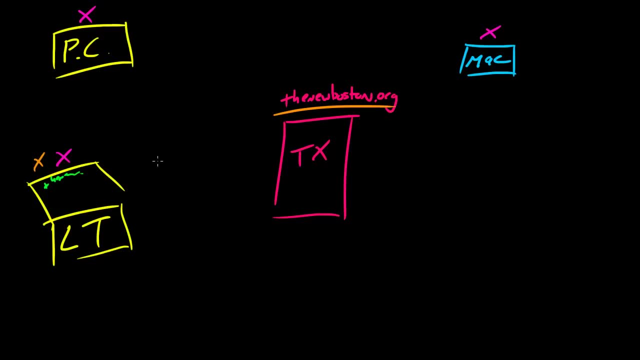 know exactly how your router knows to talk to my web server. that's a complicated process, but basically you're going to eventually get to my server right here and what your computer is basically asking is: can i see the new bostonorg? or basically, can you send me some files from this?